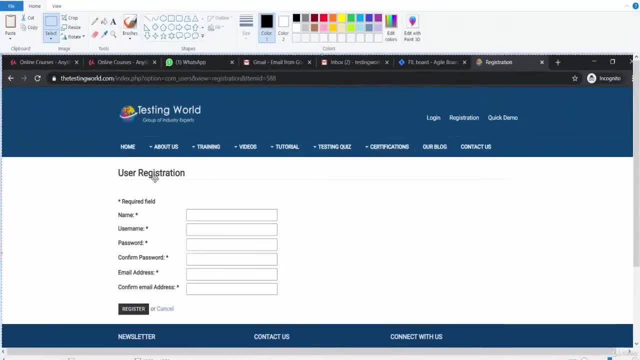 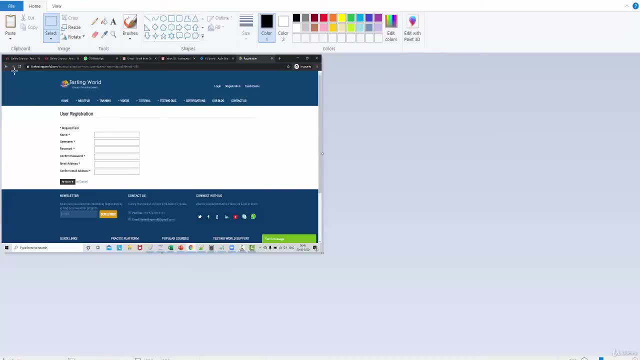 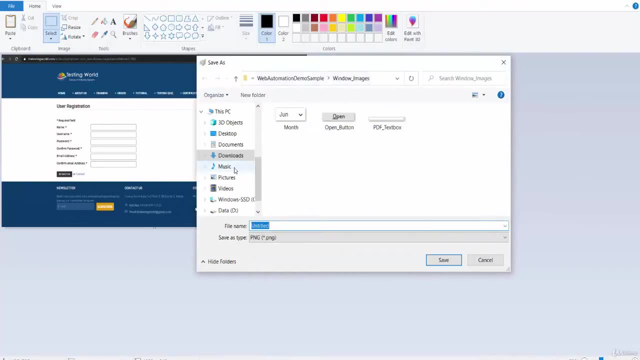 Going for MS Paint and just saving it. So I'll just save it somewhere And I'll just select the area, like I want to just keep this area, Save it on my desktop And there on the desktop we have a task folder. I'm saying Captcha missing. Okay, now, whenever you, 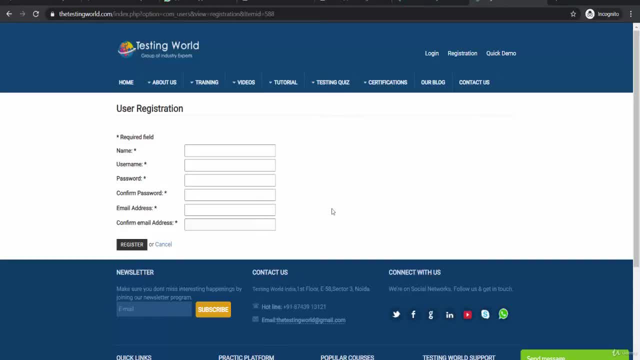 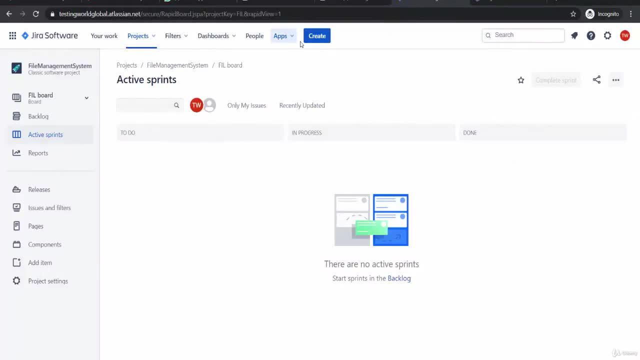 have any bug. I have just taken the screenshot of this. Now I want to report this bug into Jira, So I'll just go on to my Jira. Here we have a create button, So I'll go to create a new defect. 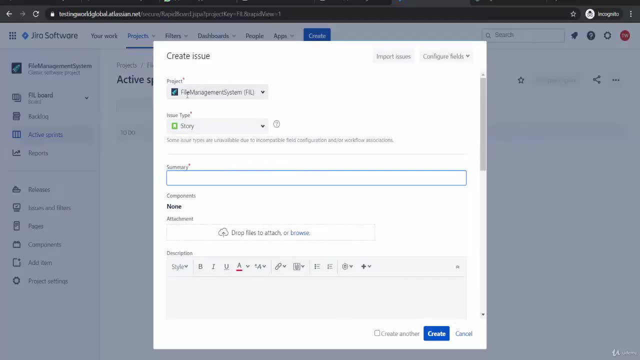 I'll just click on this create Now. first of all, it is showing me the project. Now I'll explain many fields which we are having on this form. Okay, First of all, we need to select the project on which we are working. 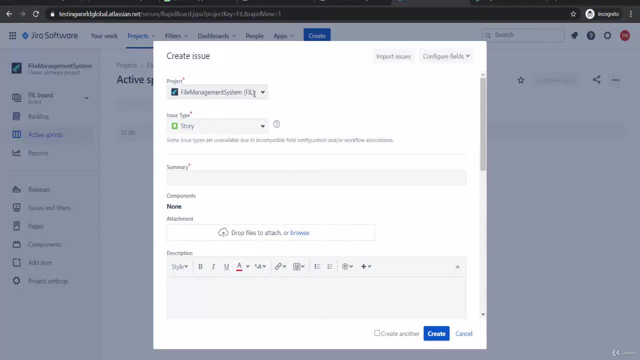 As of now, I am allocated to one project only, So in this dropdown it shows only one project. But it might be possible you are allocated to multiple project, So you will get different project. You need to select the project to which you want to report this defect. 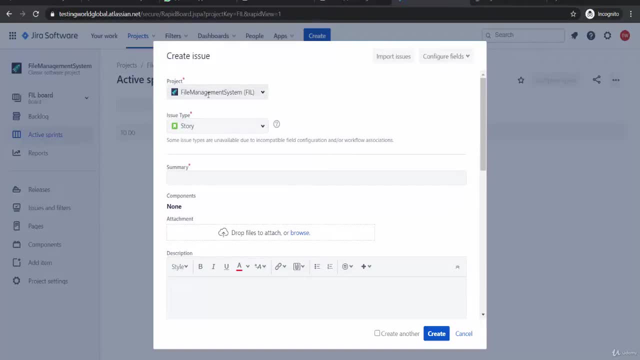 But as of now we have only one project, so I'm just keeping it same Now. next I'm coming to issue type, So I'm going to report a defect here, or I'll say bug. I'll just go to the dropdown and select bug. 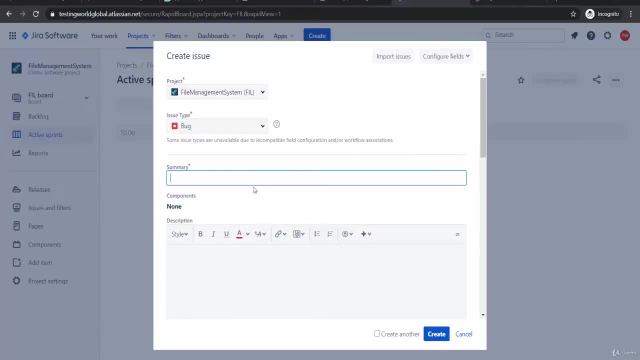 Now next is summary. We need to fill the summary information here. Summary means a basic information about the bug. So here we need to give information about the bug in minimum number of words. So I'm saying capture is missing on registration page. Here, in the summary field, we need to give information about the bug. 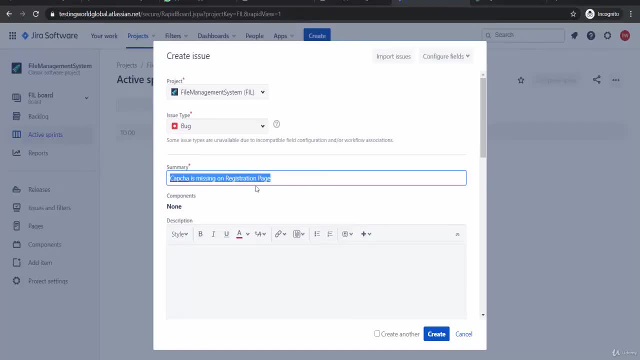 With minimum number of words, and it should be clearly understandable to anyone, Because in most of the cases people will see the summary only and will try to understand this bug. So here it should be understandable. line with minimum text. Okay, next I'm coming to description, which is very important. 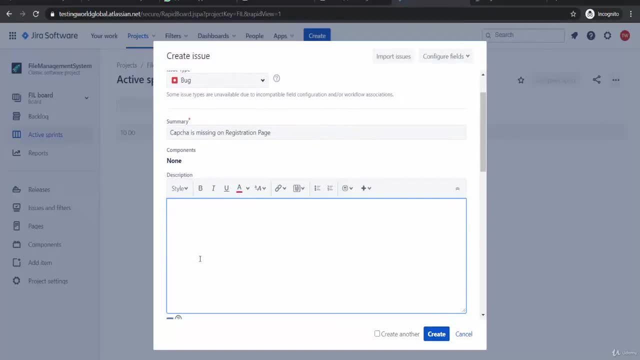 In the description we need to describe complete defect or I'll say complete bug. So here in the description I'm just writing like, while testing registration functionality on registration page we are not getting capture Image And text box- Text box to enter capture data. 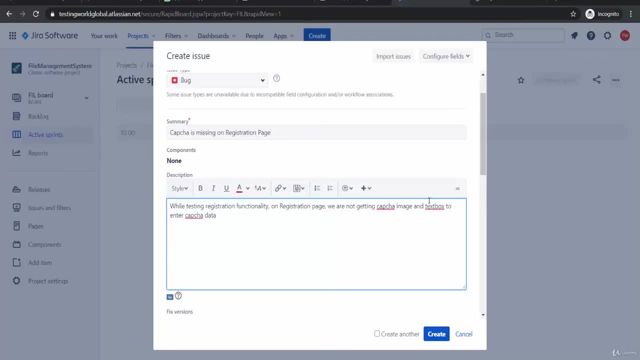 To enter capture data. So we are not getting that Okay here on this page. expected is that capture image should display user should be allowed to register. Okay, So I'm saying actual result only after filling correct capture information. So that's my expected value. 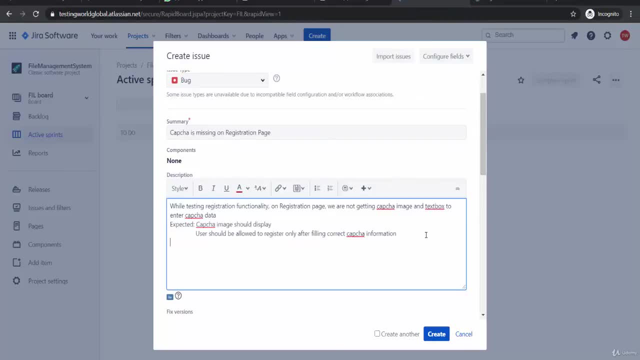 Means in this case that should be the expected value, But what actually is happening? So I'm saying actual result: capture is not on the page. User is not on the page. User is allowed to register without capture. Now we have given this information and I would suggest you can use these options to. 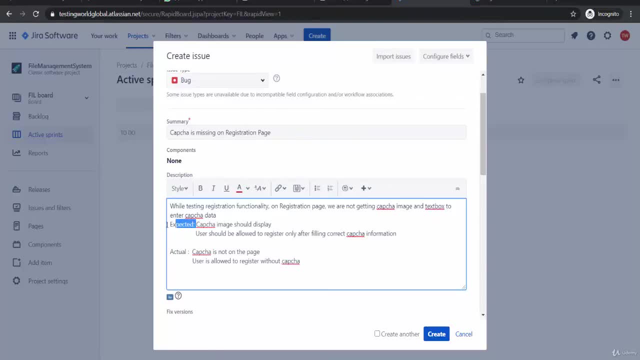 highlight the information. So I'm saying, okay, expected, I want to make it bold, actual, I want to make it bold. Apart from it, this, These two lines. I want to display red color text. So I've just selected that. 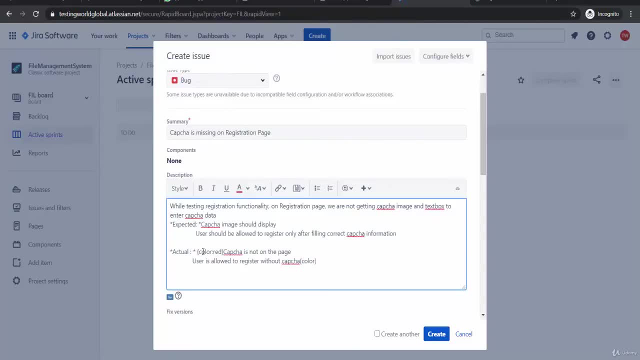 Okay, Now my description is there. Normally, when you're writing description, we need to give detailed information, So here I'm giving the information in detail. Okay, One more thing you can put here is steps to reproduce, Because here on this form, you will not get any other area to put steps to reproduce. 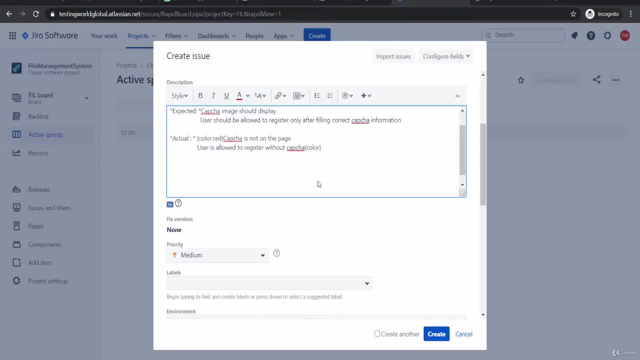 What do you mean by the steps to reproduce? Steps to reproduce, Steps to reproduce: Okay, What steps you have to follow to replicate this defect. So I'm saying, okay, steps to reproduce. What? all the steps you need to follow? 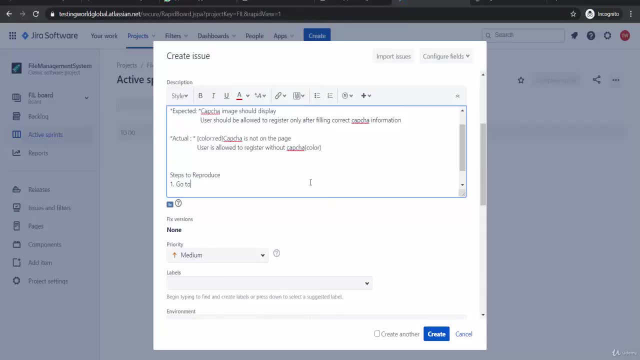 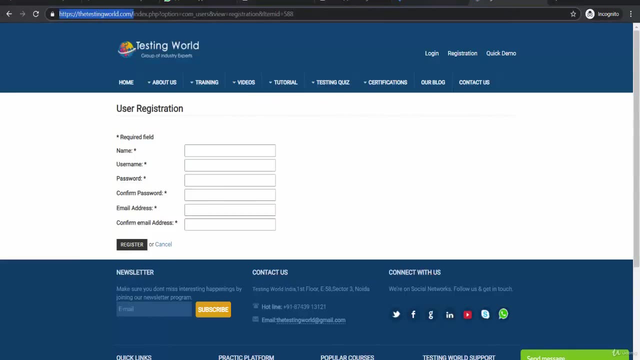 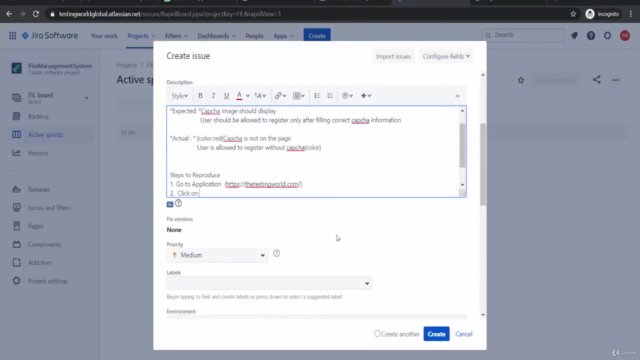 So I'm saying, go to application And if you want you can pass information like that's the URL. You need to go to this URL. Okay, Now step two: Click on Registration link on top right corner of the page. 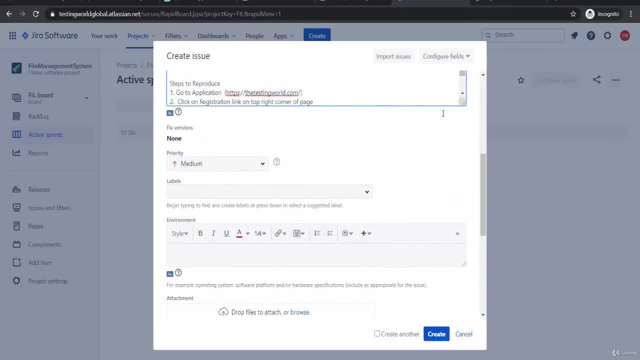 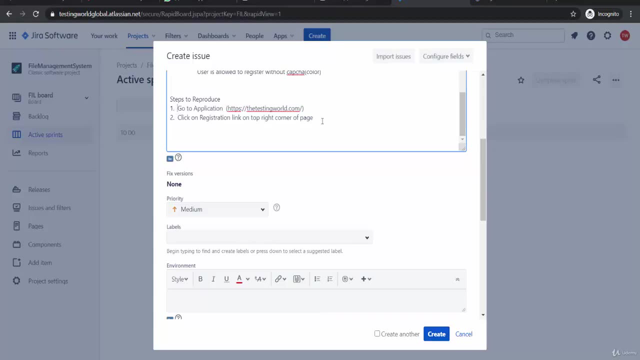 Of page. So here we need to write as many steps we are having. As of now, we have only two steps. I'm just keeping it two, But you can have any number of steps. Okay, After that we have actual and expected. 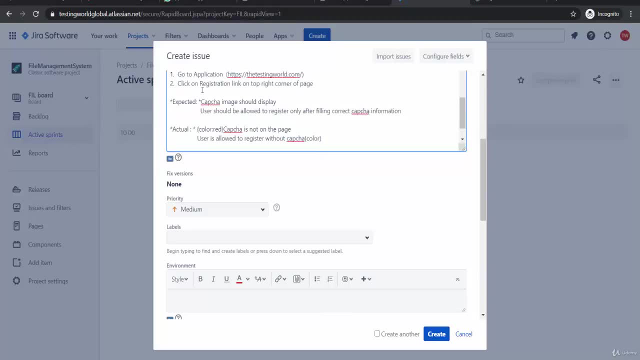 So I'm just putting the same actual expected here. Expected Once you go to this page. we should get capture and user should be allowed to register only after filling capture. But here this is happening. So I'll just put actual and expected here, with the steps to reproduce as well. 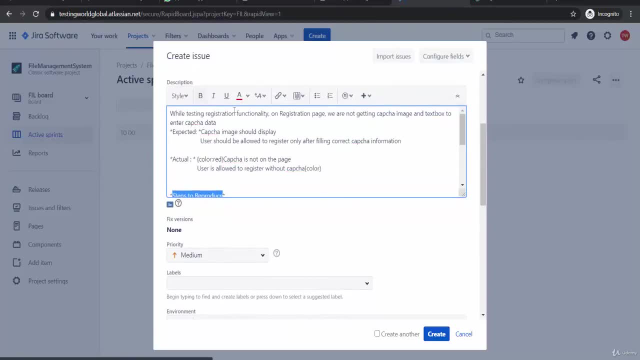 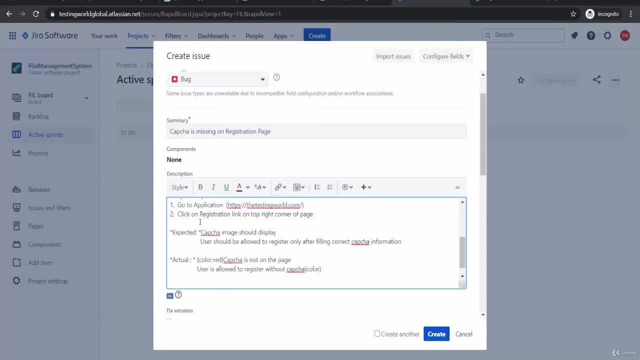 And I want to make it bold, So I'll just select bold. So that is here. in the description field, we need to give the complete description about the defect. Also, it always a good practice to put steps to reproduce. So that I've done. 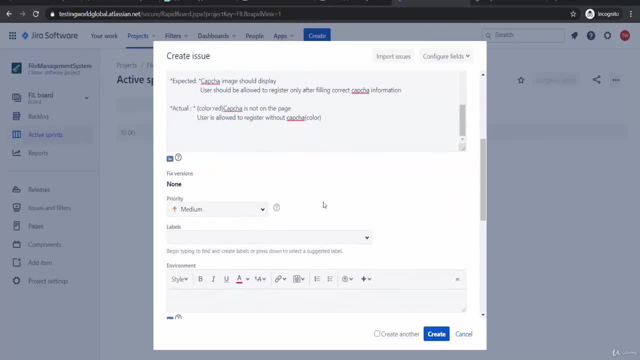 Okay, Now I'm moving to the next step here: priority, which is important. So if you're working as a software tester, I'm sure you are aware about how to decide priority. So whatever the priority you want to give, you can just give it over here. 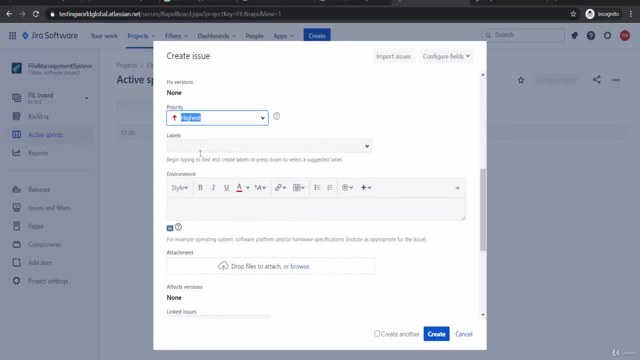 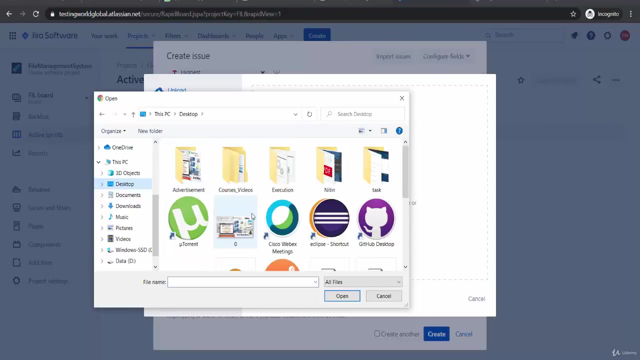 So I'm just giving the like highest. Okay, As of now, I'm not filling this label and environment. In next video I'll show you what is the meaning of label and environment. I'm just going to attach, Okay, My image, image which I have taken. 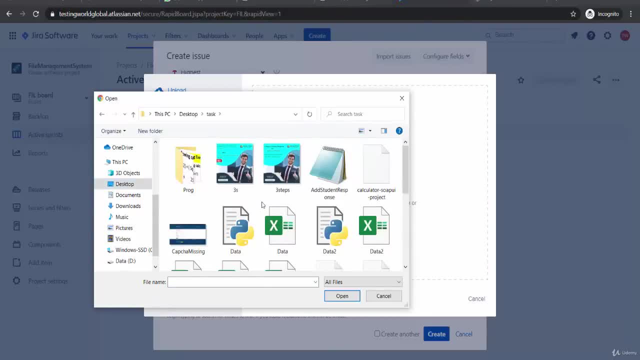 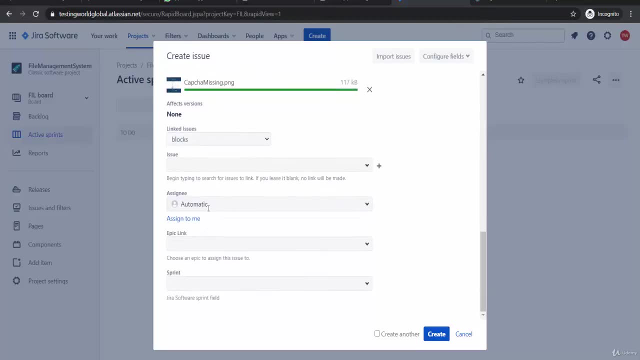 So hope you remember. we have taken an image with the name capture missing. I'll just attach it over here. I'm just coming to the next field, which is assignee. Okay, Whom you want to assign this? So as of now, if you can see, we have three users. I'm reporting a defect, but I want